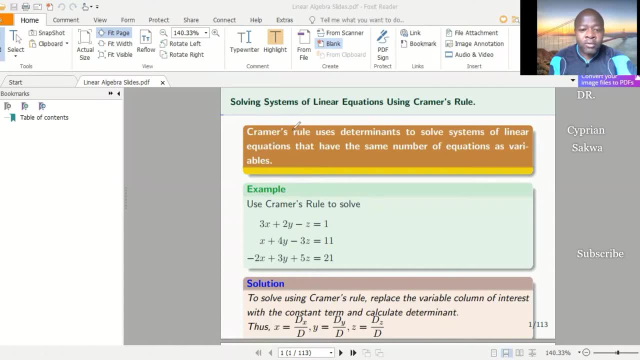 at how to solve system of linear equation by use of inverses. So today we use Cramer's rule and Cramer's rule will be employing use of determinants. So we'll be calculating determinants and then we use those determinants to calculate the value of X, the value of Y and the value of Z. So let's 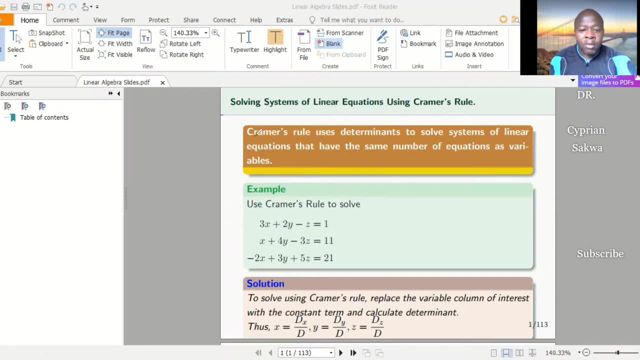 begin with this example And what you notice just before that. what you notice is that for you to solve a system of linear equation by Cramer's rule, the number of equations, number of linear equations, must be the same as the number of variables. What I mean is, for instance, in this: 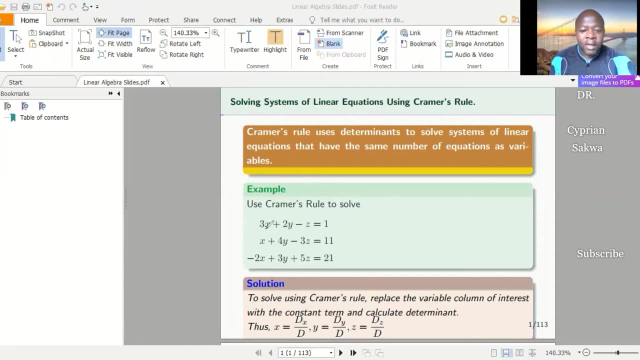 example that we're doing here. this example has three questions: One, two, three, And you really again. the variables are also three: X, Y and Z. So the number of equations and the number of variables must be equal for you to employ Cramer's rule to solve Now. so the question is: use Cramer's. 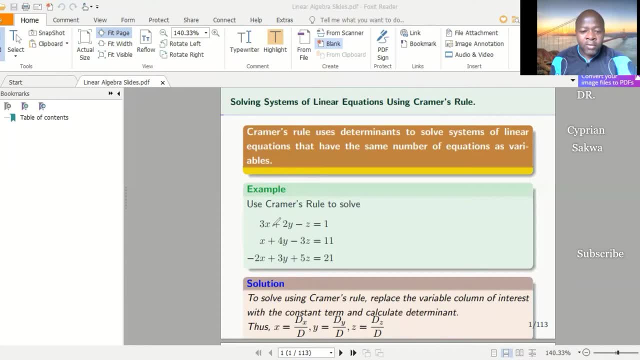 rule to solve this system of linear equation. So we'll want first of all to extract the coefficients And then, after extracting the coefficients of these equations, determine the number of variables that are within the determinants and use those determinants to get the solution. Now I've 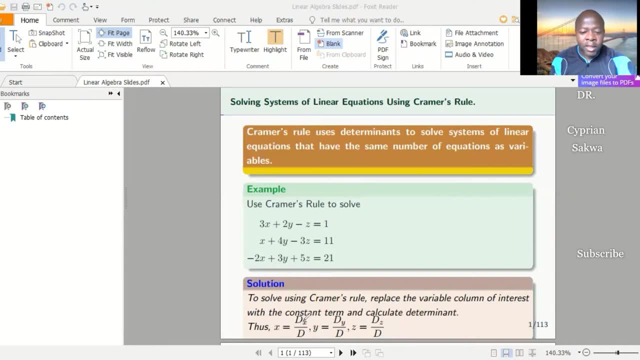 written here that thus X will be given by dx over d, where dx is just the determinant with respect to x. Now I'll show you how to get the determinant with respect to x, And then d is just the determinant of these coefficients, here the coefficients of these coefficients, right. 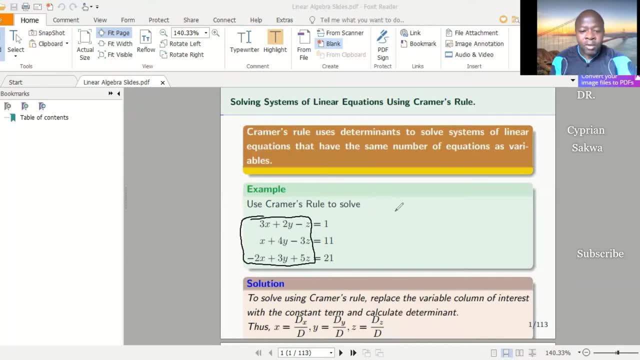 is part, so they will fit. there are three, two, negative one, we have one, four, negative three and negative two, three and five. so this determinant is what I'm calling D, this determines work. accordingly, so to find the guitar with respect to X, and notice that this column is for the coefficients of X, so this: 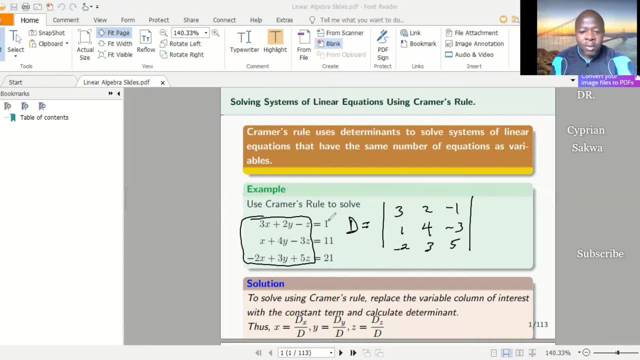 column of the version of X is what I'll substitute with the constant here. these are the constants, the concept and that's what I've written here. I've said that to solve using Kramer's rule, we replace the variable column of interest with the constant term. so the concept comes here. so the variable interest is X and the 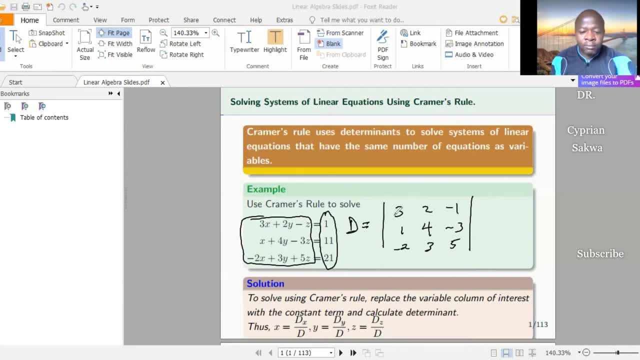 column for that X was this. so this column is the one I replace with a constant, and that means, therefore, that for me, to find the determinant with respect to X, it's this column that I have to to substitute with a constant. the cosine is 1, 11, 21, and so 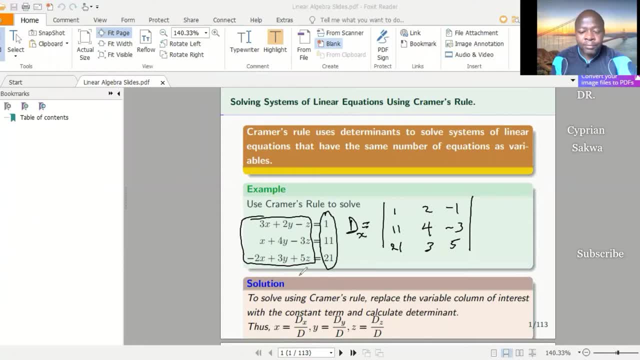 that will give me the determinant with respect to X, DX. so if I want the determinant with respect to Y, I replaced this column of Y with the constants, and the other column means the other column of the value. so let's look what this example and how it's done. 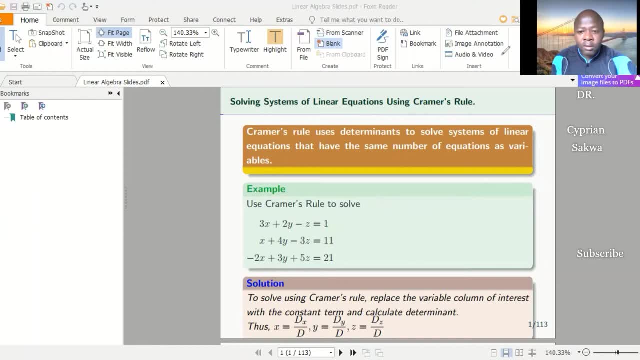 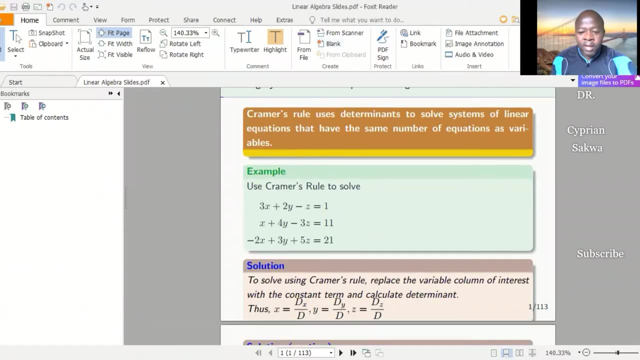 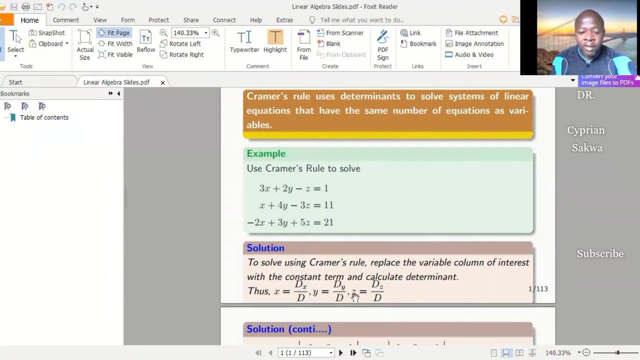 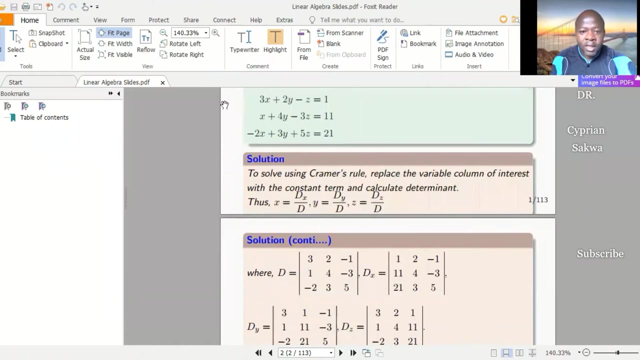 the question is used famous rule to solve this and the world said that we want to find an excellent answer. because this x, then divided by d, then we divide by d to give us the value of y, then it is z divided by d shall give us the value of z. let's write the coefficients, so our d, as we've already stated, 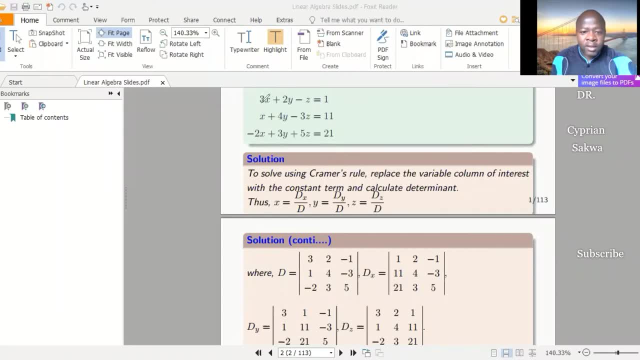 our d are the coefficients of this, that's three, two negative, one, one. four negative, three negative, two, three, five. so this is our d. then we do x, we only replace the column of x. so the column of x we replace with the constant 1, 11, 21. that's what you see: 1, 11, 21. the rest remains the. 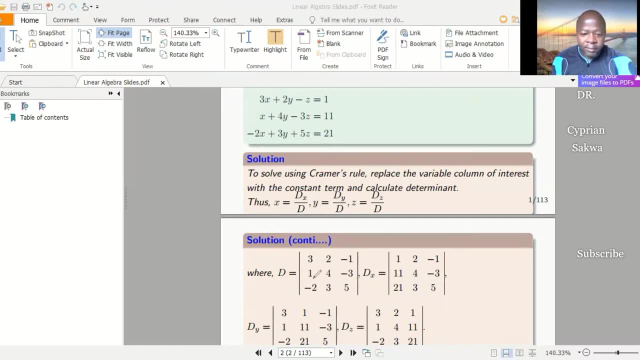 same. and then we come to find the, the terminal. with respect to y. that means we'll be replacing the constant of y column of Y. So I'm using this D. So on this D I just replace the column of Y. So the column of Y I replace with this constant. 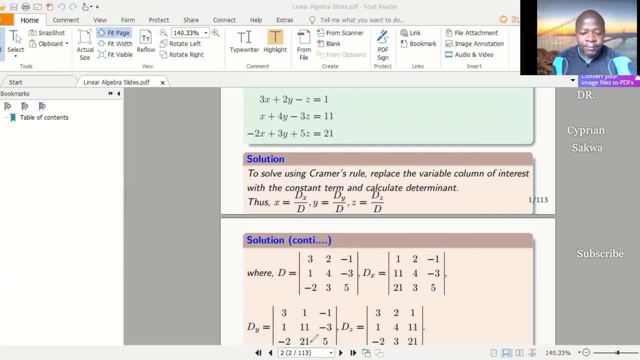 1,, 11, 21, So the rest remain. the column with the x remain. I replace the column of Y, the column of Z remains, and then I also want the determinant with respect to Z. that means the first two columns remain the way they are. 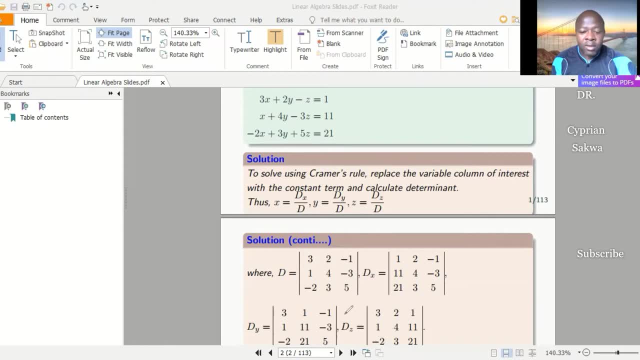 the first two columns remain the way they are, but now this column with respect to Z, this column with respect to Z is the one I replace with the constant 1, 11, 21, 1, 11, 21.. And you can see that I put them. 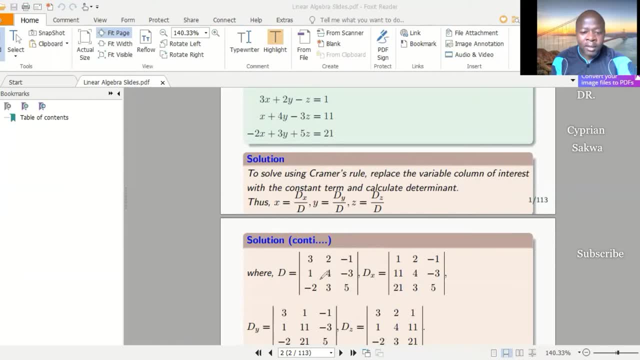 inside these parallel lines. These parallel lines means determinants that determine the determinant of this, determine the determinant of that, determine the determinant of this, and so on. Now, so far, we know how to find determinant of a 3x3 matrix. In our previous video we looked at that. 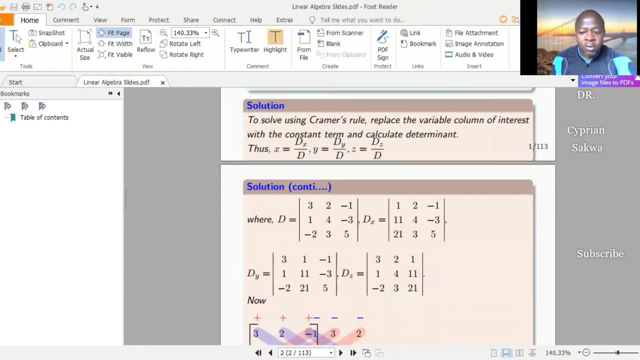 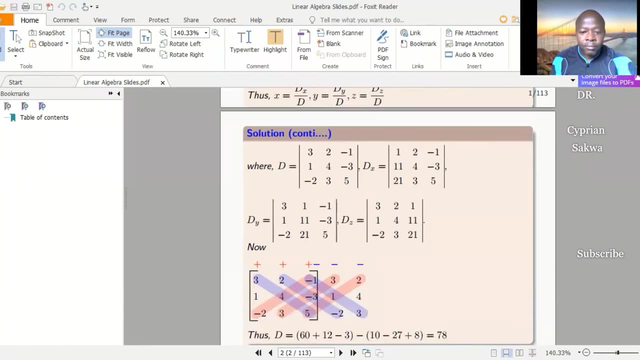 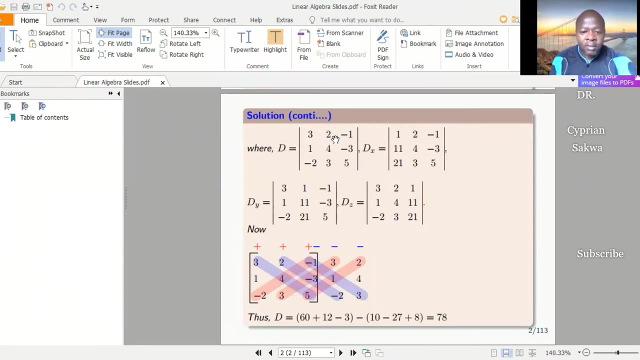 So we'll go straight to determinant. I'll use the simplest method that I showed you in one of my videos. So I want the determinant D. So you can see, this matrix is the one I've written here. This matrix of D is the one I've written here. 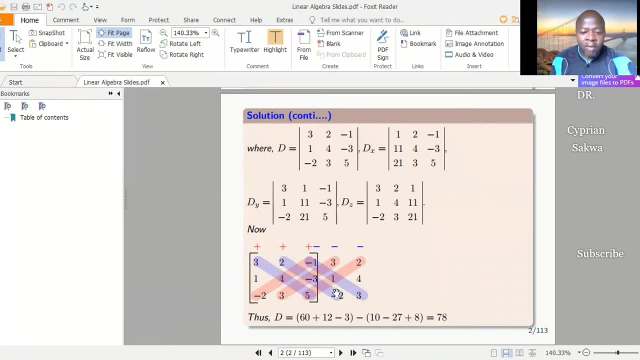 So these two columns, the first two columns, I have added them here. I've added them here. So this method I've shown you before just repeating it. So you realize that there is a column, there is a diagonal running from the top left to the bottom right. 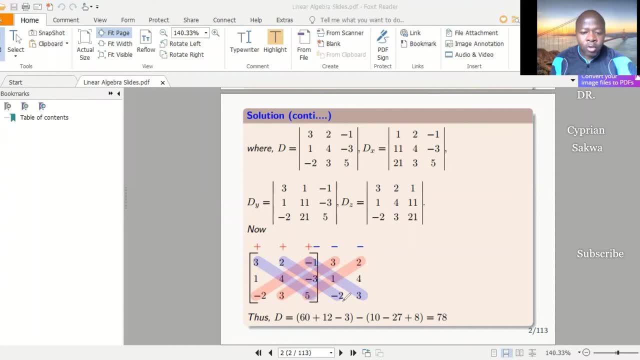 There are these three diagonals in blue running from upper left to bottom right. So we multiply along these diagonals and add the results. So you can see: I multiplied 3 times 4 times 5 to give 60, 2 times negative 3, that is negative 9. 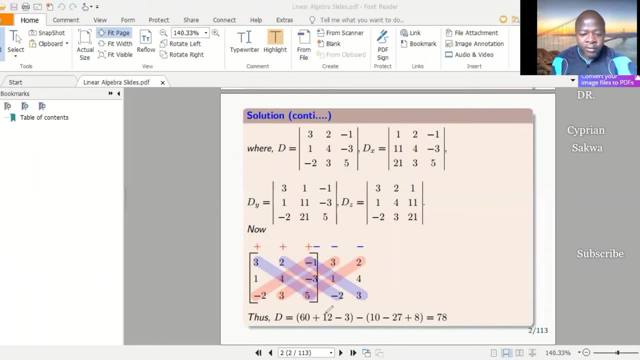 now negative 6 times negative 2, and then this other one, negative 1 times 1 times 3, gives negative 3.. So I've multiplied along these three diagonals and added the results. Then I say minus. This time multiply along the diagonals in red. 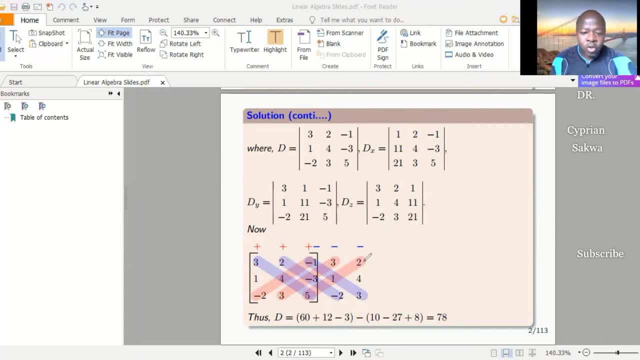 the diagonals in red running from top right, top right to bottom left. So, for instance, 2 times 1 times 5 is 10.. So I multiply as I add the results 3 times negative. 3 is negative 9 times 3, that is negative 27. 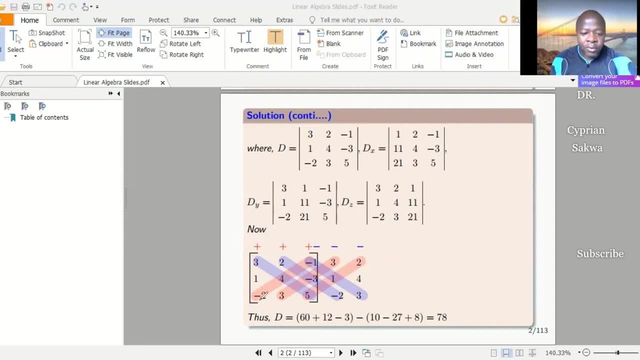 and then this other one, negative 1 times 4 times negative, 2 is 8.. So I add the results in the first bracket, add the results in the second bracket and subtract the two results, I get 78. So 78 is our. 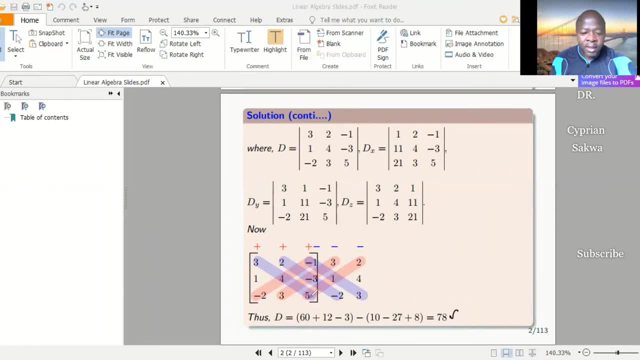 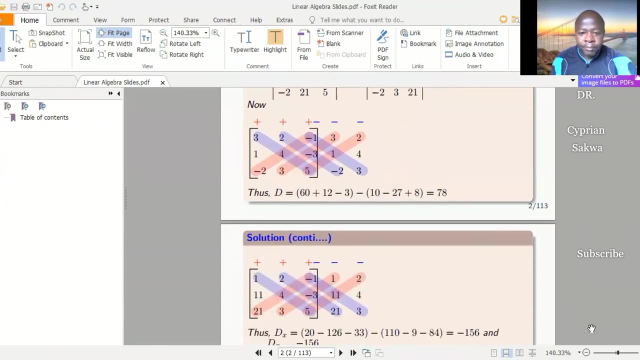 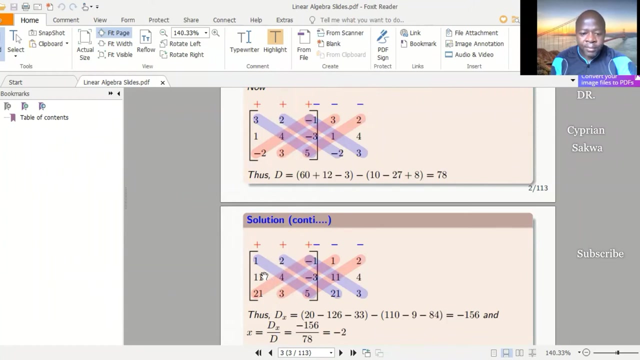 D. The determinant D is 78. So I do the same for DX: Define the determinant with respect to X. So I've done that in the next page here. So what you see here is the matrix of DX, Matrix in DX I take the two. 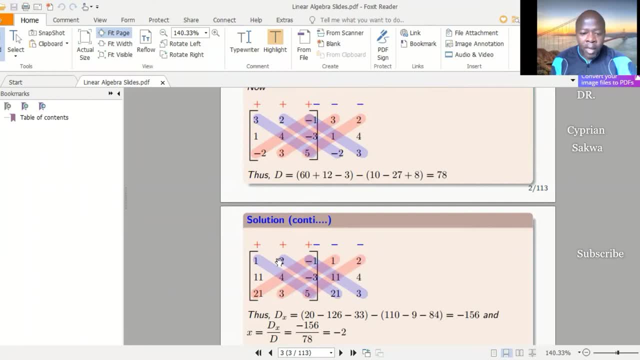 columns and add them here. Multiply along the blue diagonals as I add the results: 1 times 4 times 5 is 20.. 2 times negative: 3 times 21 is 126, and then negative: 1 times 3 is negative 33.. I add those results, Then I come. 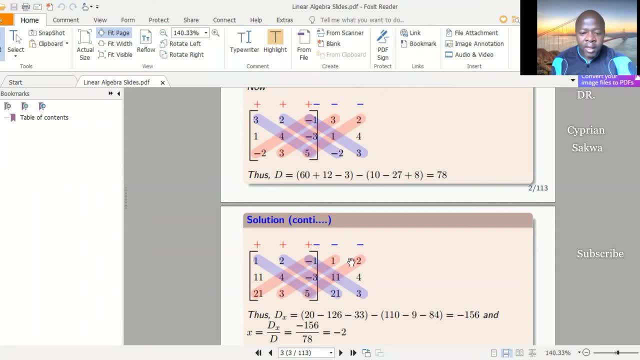 to this other diagonal in red and multiply, add the results, and the results are here. When I subtract these two, I get negative 156 and therefore I had already said that to get X I'll take DX, Because this is my DX, the determinant of this matrix, DX. 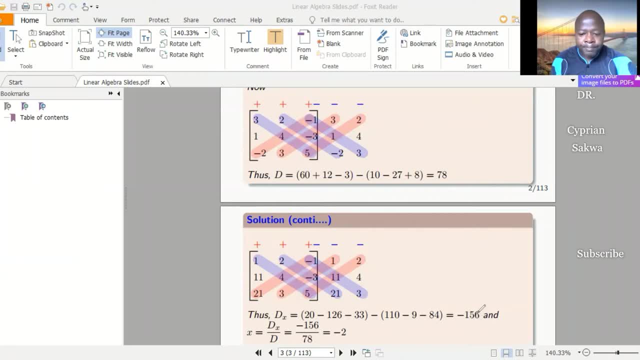 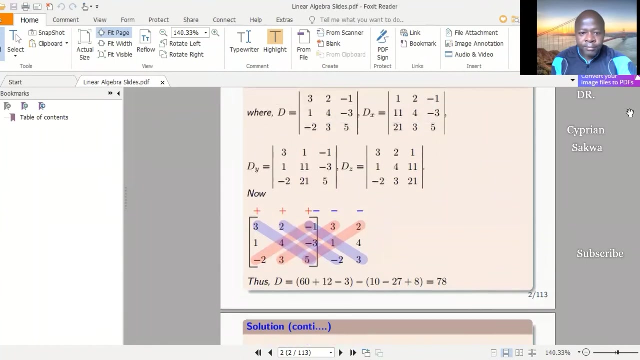 So that determinant is here negative 156.. I had said that to get X I'll take DX divided by D. So DX is negative 156 divided by D, which is 78.. That gives me negative 2. Ok, Let's go back and see what DY was. DY was: 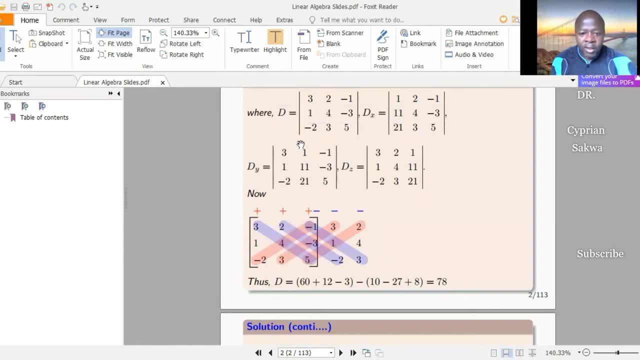 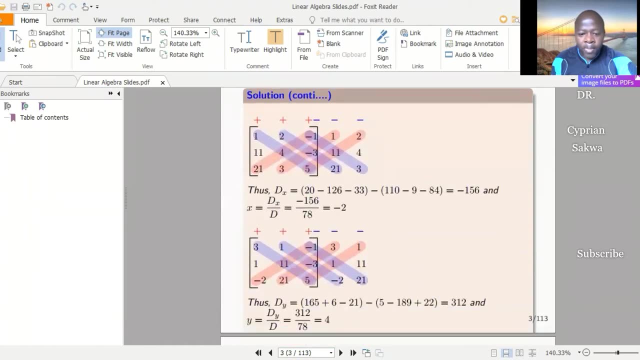 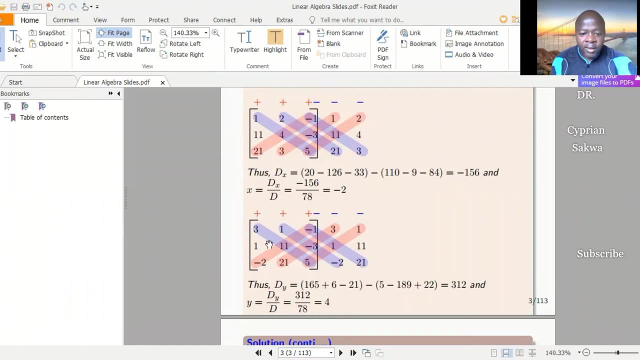 the determinant of this matrix. So I want to find the determinant of this matrix. So I found it in here. I found it here. This is our matrix, This is the matrix. Then take the two first row columns, the first two columns, Add them here and then 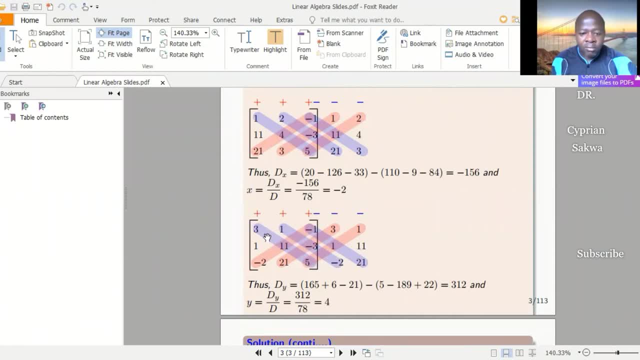 identify the three diagonals running from top left to bottom right. multiply along those diagonals and add the results. So 3 times 11 will be 33, times 5 will be 165.. Multiply along this other diagonal to get positive 6.. Multiply along this other diagonal to get. 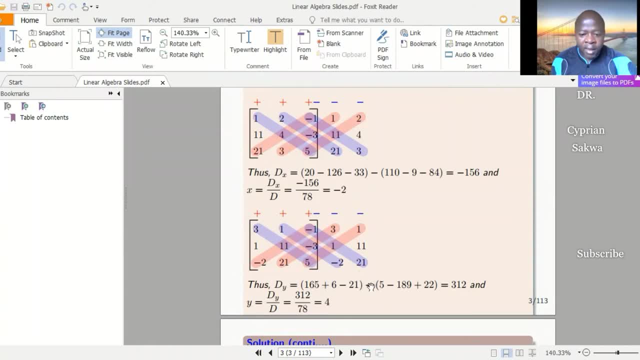 negative 21.. Add that result, Then minus Multiply along the diagonals in red. That is 5 times 1 times 1, which is 5, and this other one will give you negative 189, and this other diagonal will give you positive 22. 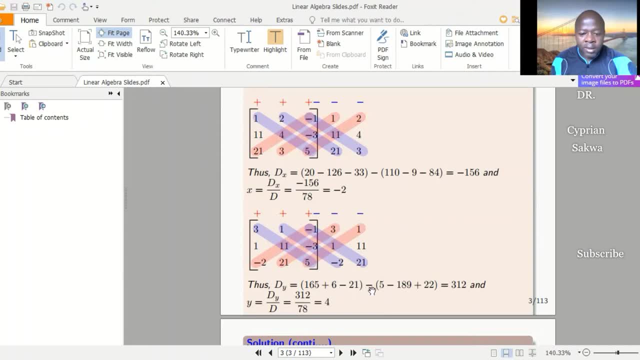 So when I do this, add the first bracket minus the result in the second bracket, I get 312.. So what is Y? Y is there for DY over D, which is 312 over 78, and that gives me 4. So I do the same for Z. 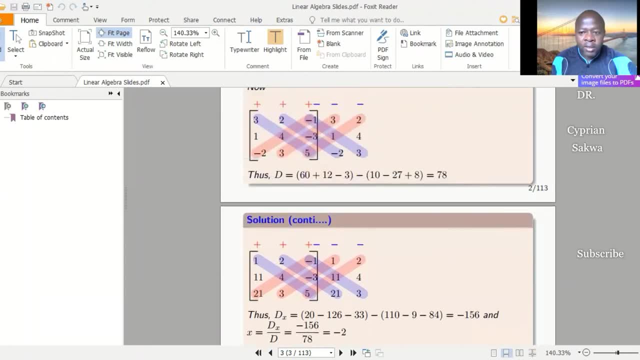 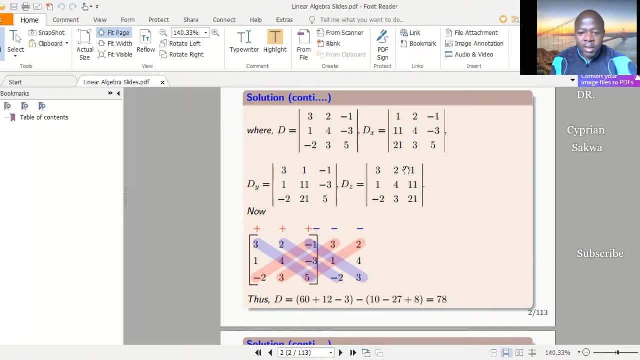 I do the same: to get Z, I come back. There was a Z here, I come back. There was a Z here, I come back. There was a Z here. I want to get the determinant. I want to get the determinant, This determinant, This determinant. 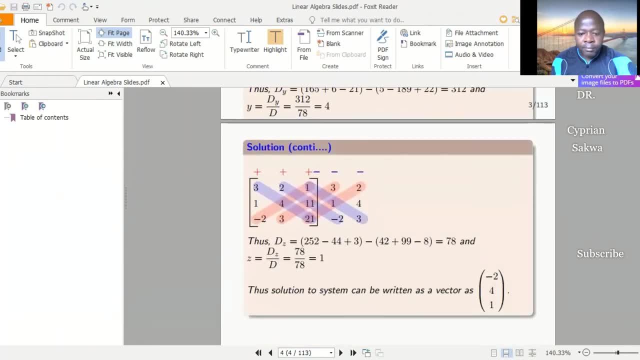 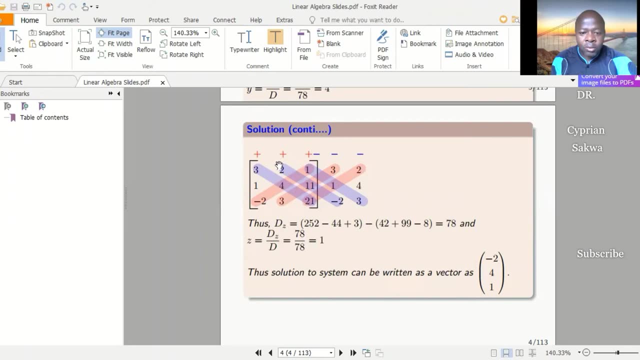 So I come here. So I come here. This is the matrix. This is the matrix. Take the first two columns. Take the first two columns and add them here and do what you have been doing: multiply along the blue diagonals and as you add the results, you get 42 minus 44 plus 3. 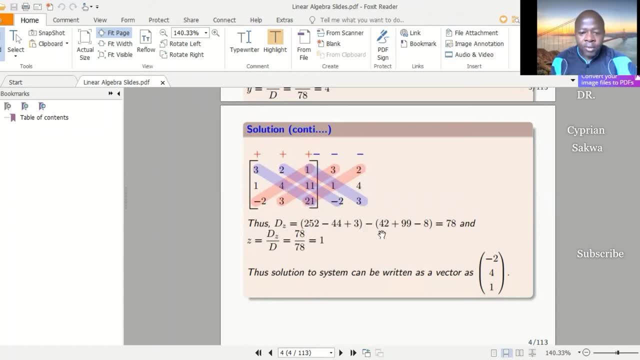 then multiply along the red diagonals. then multiply along the red diagonals, you get 42 plus 99 minus 8. you get 42 plus 99 minus 8. Now this first bracket minus the second bracket, Now this first bracket minus the second bracket, the answer is 78. 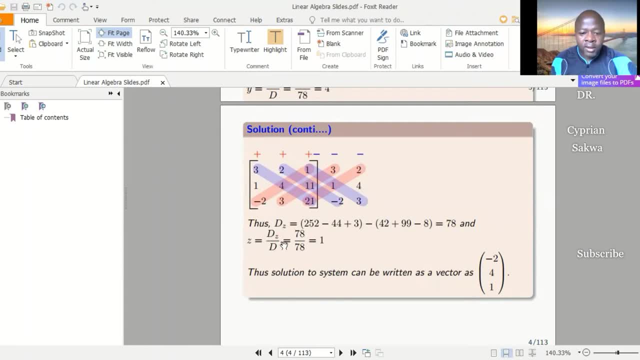 So Z is DZ over D, which is 78 out of 78. that gives us 1. So we now have the value of X, Y and Z. So what is the solution to the system? We say the solution to the system shall be written in vector form. 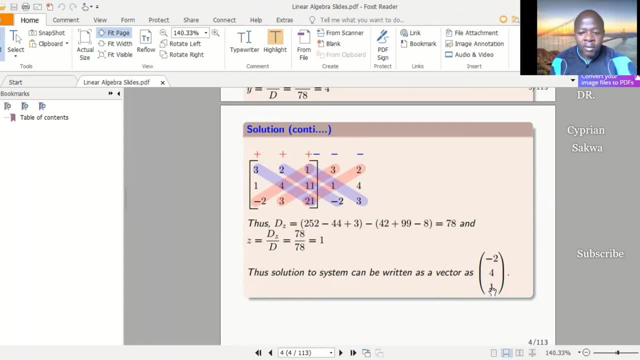 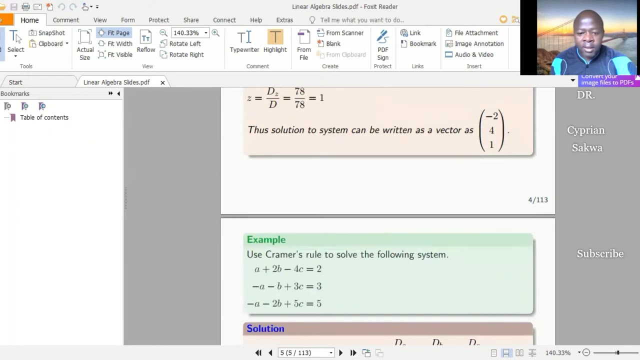 the value of X, the value of Y and the value of Z. So this is the solution to that system. Let's pick one more example, Let's pick one more example, Let's pick one more example, and then we see, so that we can master how to use Cramer's Rule. 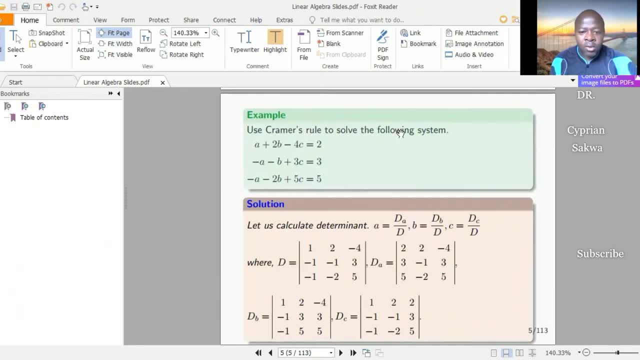 An example is Use Cramer's Rule to solve the following system: is A plus 2B plus negative, 4C is 2. So you can see the system, that it has two equations and the variable. no, it has three equations and the variables are three. 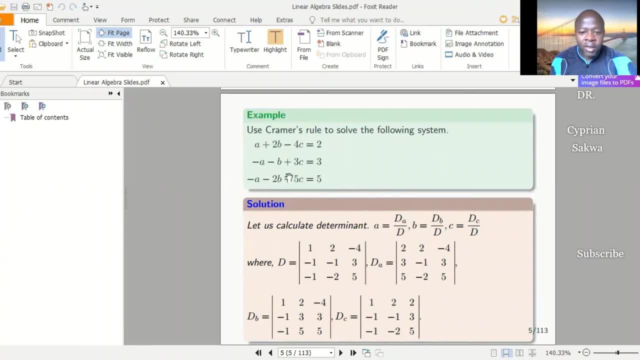 So since the number of equations and the number of variables are the same, Cramer's Rule can be employed. So we know that, to get A, we know that, to get A, we shall take dA out of d. to get B, we shall take dB out of d. 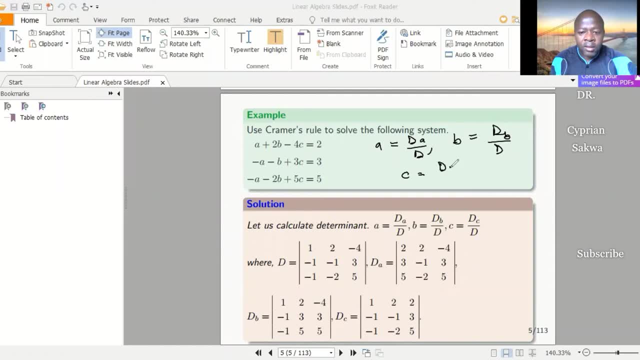 and to get C, we shall take dC out of d. So what is interesting here is how to get dA, dB, dC and d. So we just repeat the same process: that d shall be the determinant of the coefficients that we are seeing here. The coefficients here are: 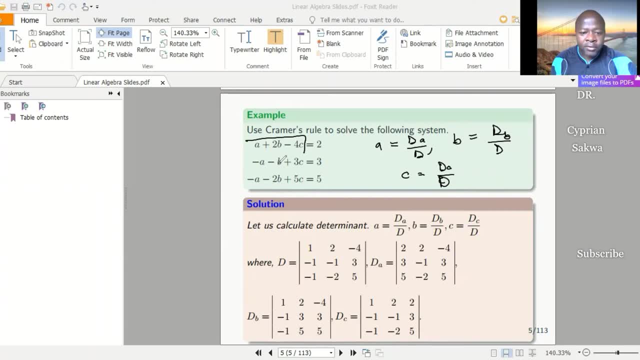 1, 2, negative 4, negative 1, negative 1, 3, negative 1, negative 2, 5, and that's what we are seeing here. that is the determinant that gives us d, and then to get the determinant with respect to: 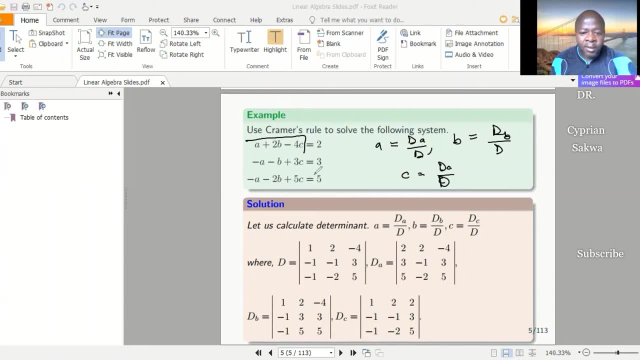 A. we shall replace this column of A with the constant column 2,, 3,, 5. that's what we are seeing here. 2,, 3,, 5 and the rest of these columns remain the way they are. and then we come to find the determinant, with respect. 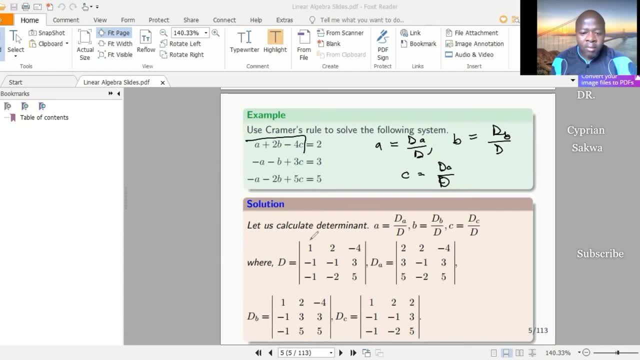 to B. so the rest, the column of A, remains, the column of C remains, but this column of B, we are replacing the constant 2, 3, 5. 2, 3, 5. and then what is dC, the determinant with respect to C? 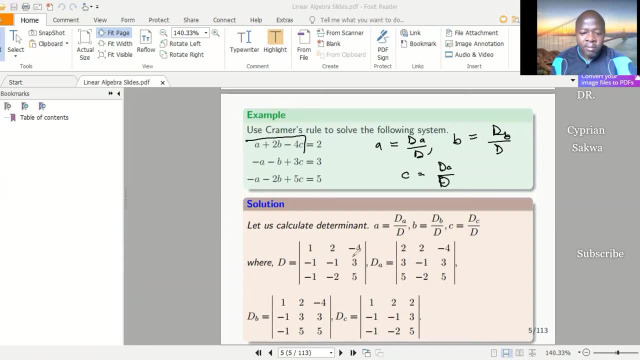 so the column of A remains, the column of B remains, but this column of C is the one that we substitute, we replace with this constant column, and that's what we see here. so we now come straight to determining the determinant. this determinant d, dA, dB and dC. 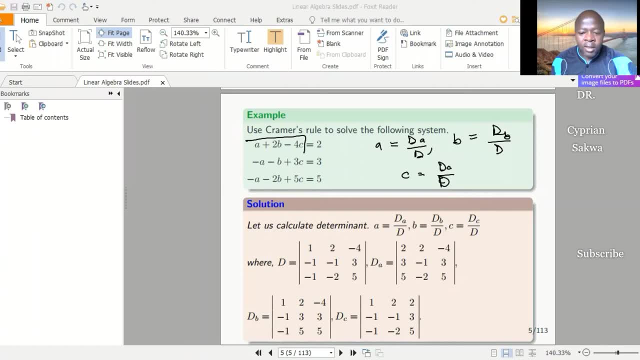 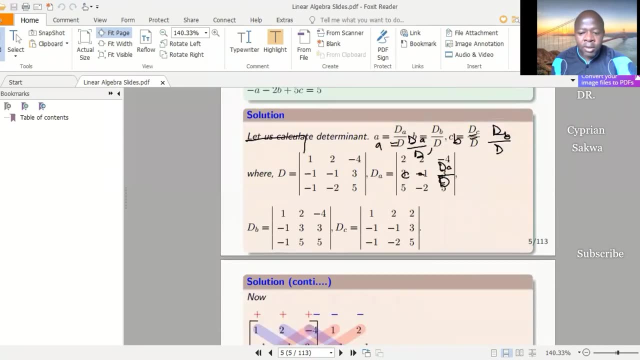 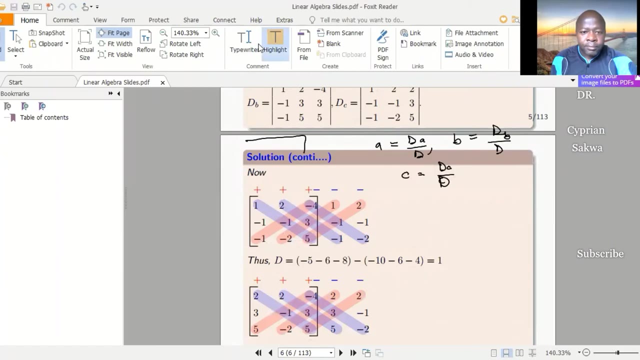 and there are so many ways of doing calculating the determinants. so, since these are 3x3 matrix, let me use the same method that we used in example 1, just a minute. let me replace that now. so this was our d. take the first two columns. 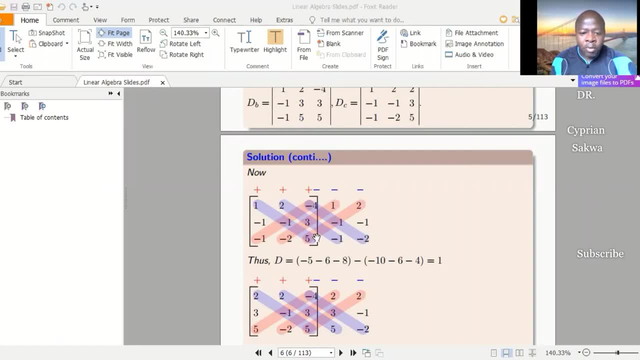 and add them here and multiply along the blue diagonals, write your result in the first bracket and then multiply in the red. now this red, these are diagonals. multiply along these red diagonals and write your result in this second bracket. so, for instance, this would be: 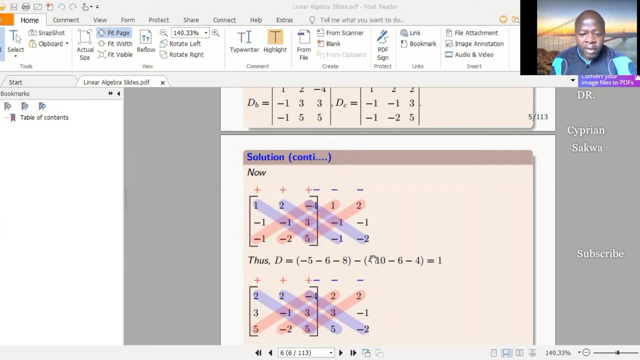 two times negative. one times five, that will give us negative ten. and then one times three times negative, two, that will give us negative six and negative four times negative. one times negative, one, that will give us negative four. so when you do this, you find that your d is one. 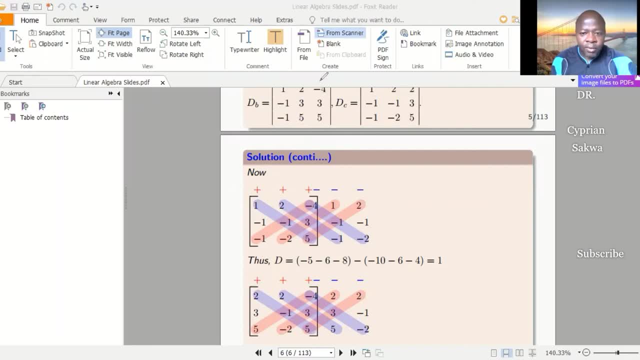 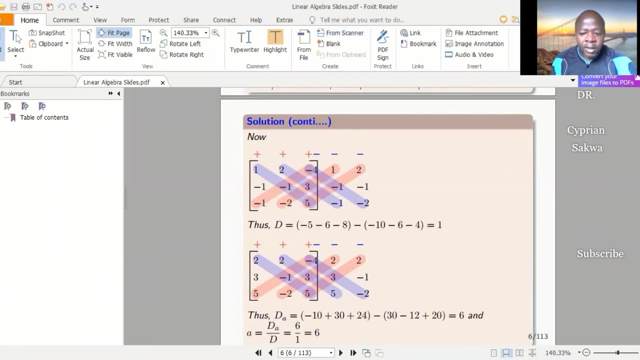 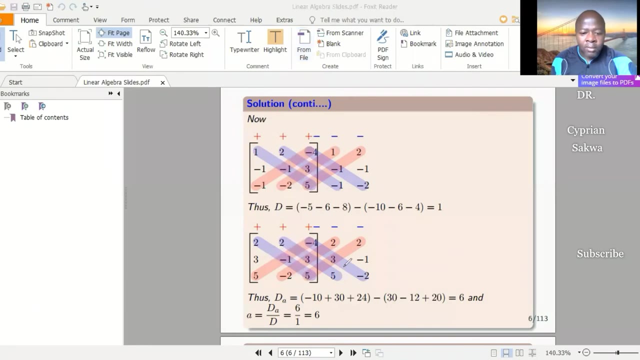 what about dx? take the first column, take the matrix that was given us, the determinant of dx, and that matrix is what I have written here, the one in bracket, the first two columns, add them here and multiply along the blue diagonals. for instance, two times negative, one times five. 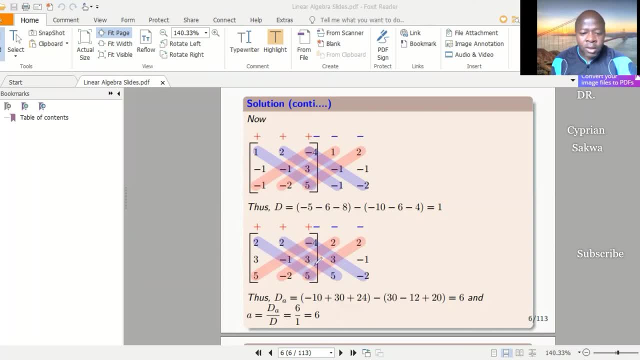 that is negative ten two times three, six times five. thirty negative. four times negative. twelve times negative. two is positive twenty four. write that result in this first bracket, then, minus in the second bracket, write what you get when you multiply along the red diagonals. when you do this: 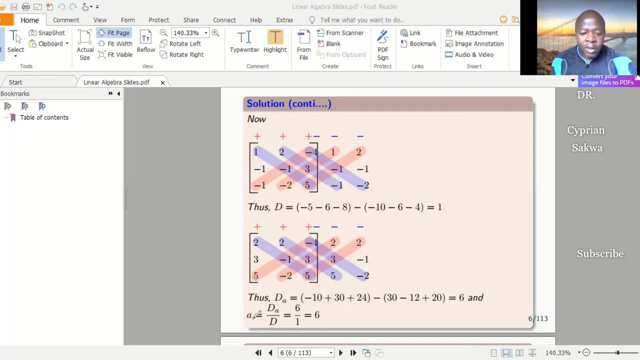 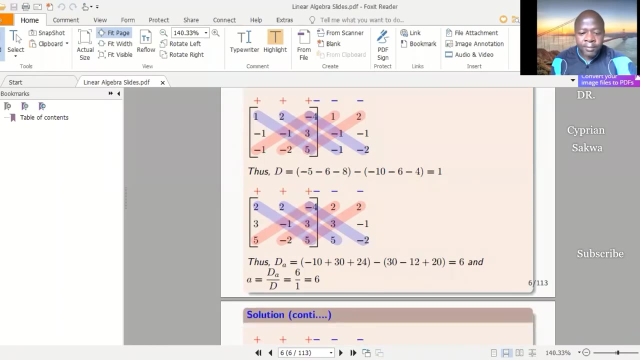 you get six as the determinant with respect to a. so what is a, a is d, a over d, that is six over one, that is six. let's proceed to find the determinant with respect to b, that is d b. so the matrix there, the matrix there was. 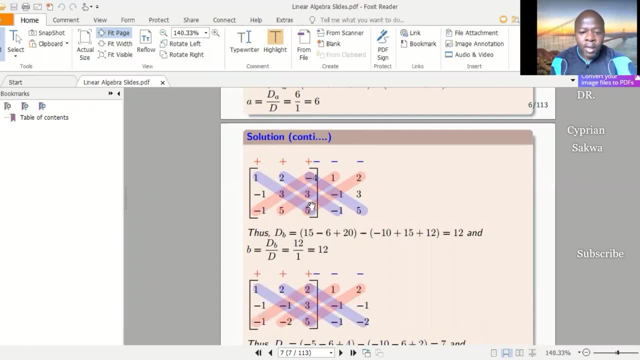 this one in bracket. multiply along the blue diagonals and write your result in this first bracket. multiply along the red diagonals and write your result in this first bracket. now i'm going through very fast in determining the determinants, because i had already gone through this. 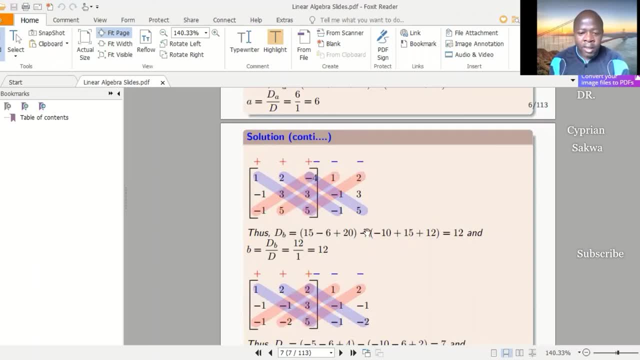 in our earlier video i already showed you how to find the determinant of matrices. so when you do this, you find that d, b is twelve. so what is b? b is d, b out of d, which is twelve out of one, and that gives you twelve. we do the same for 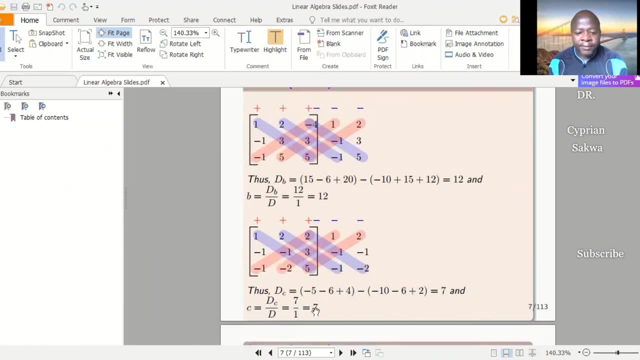 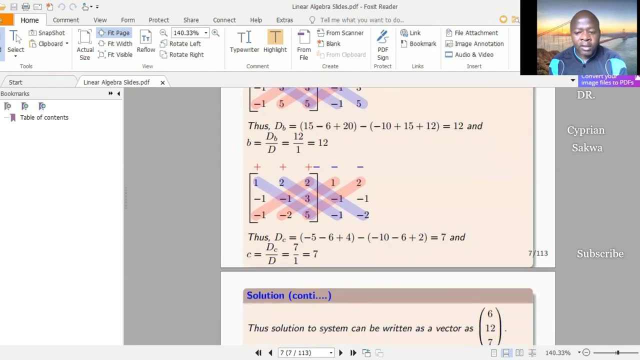 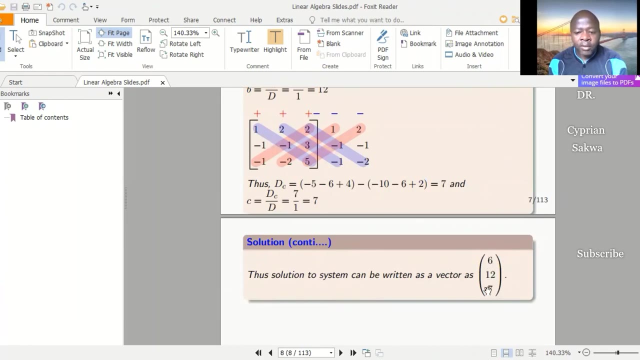 and when you do that you find that your c is seven. your c is seven. so you have the value of a, the value of b and the value of c and therefore the result, the solution of that system is written in vector form as six, twelve, seven. so six is the value of x. 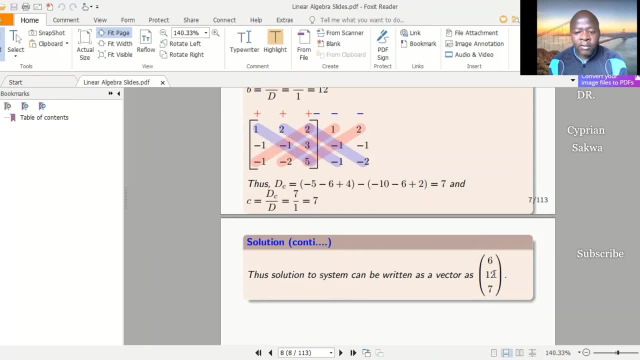 no, the value of a, twelve is the value of b and seven is the value of c, and that is how we solve the system of linear equations by Kramer's rule. so i have been loading other videos. that means that if you have not subscribed, you can subscribe so that when 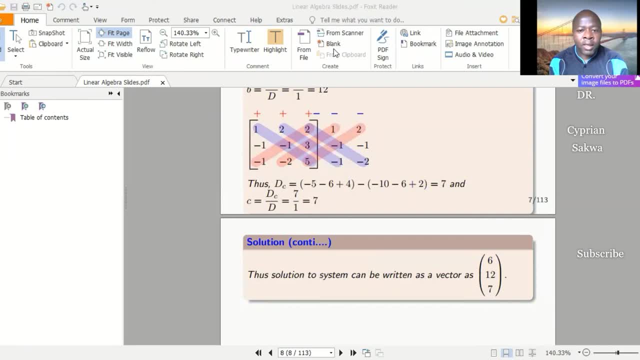 i load a video, you can automatically see it, thank you.